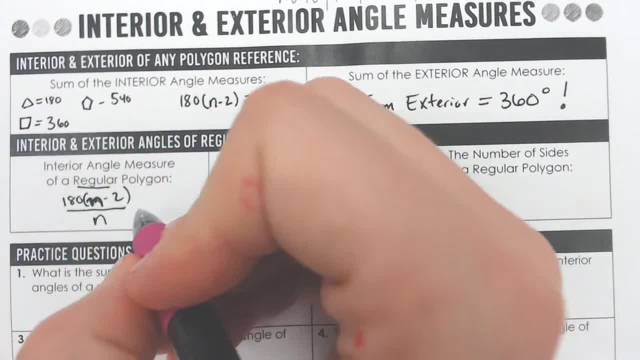 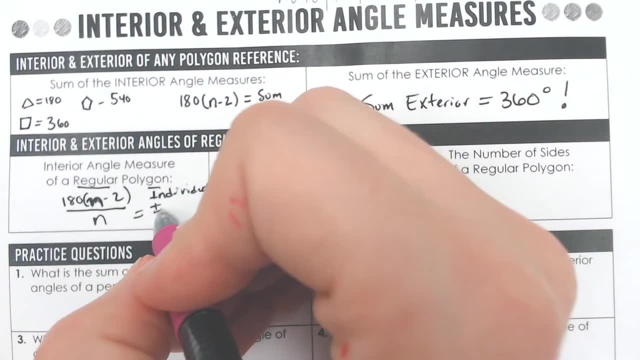 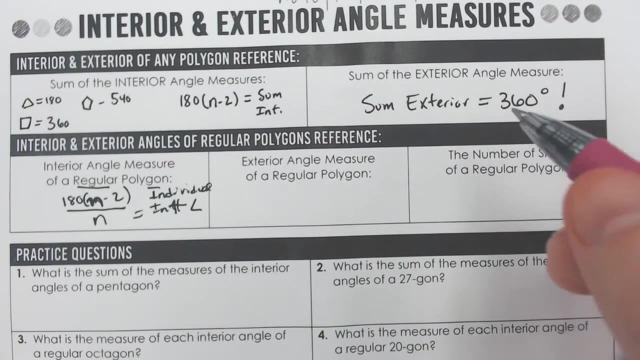 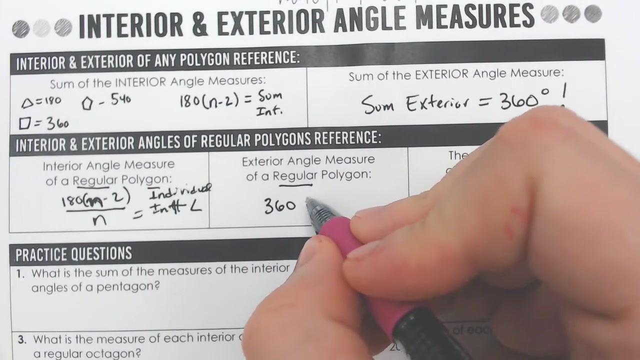 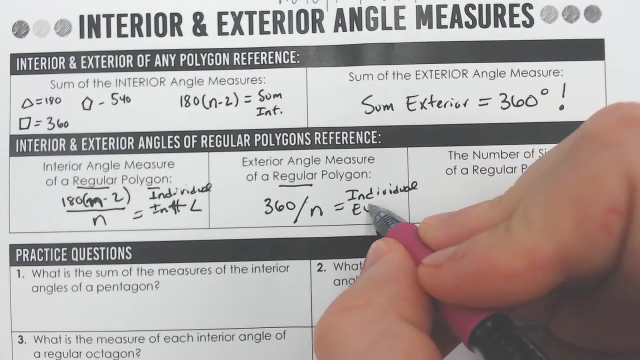 and then take it and divide by however many sides you have, and that would be a individual, not the sum. interior angle. boy, I spelled those a little sloppy, I'm sorry. the exterior angles of a regular polygon is just 360 divided by n would be the individual exterior angle. 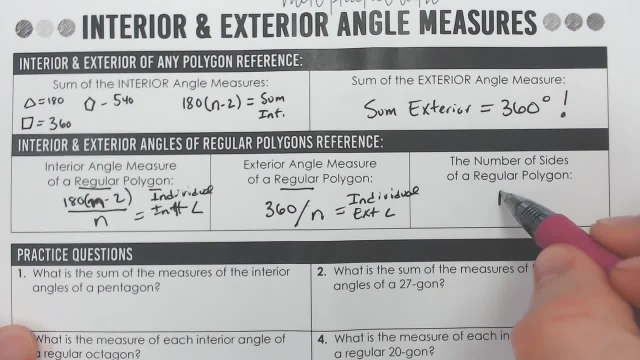 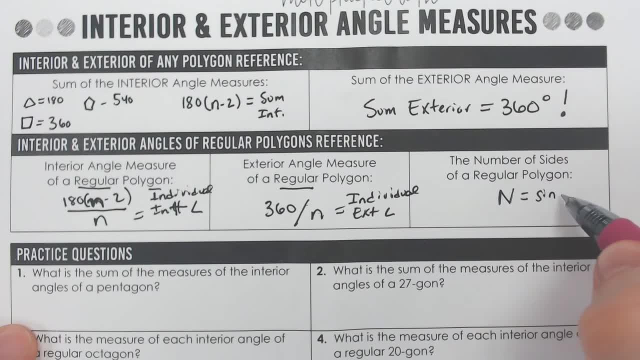 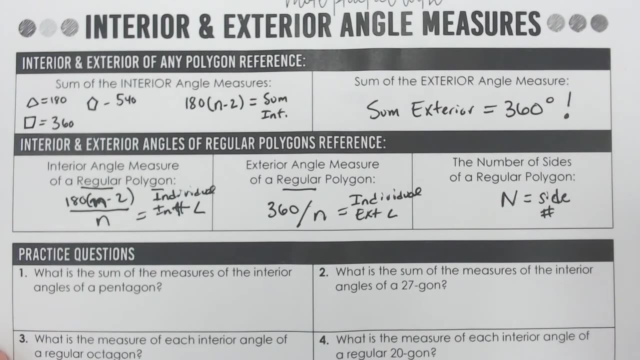 and the number of sides of a regular polygon is called n. okay, so that's? that's just representing n is equal to the number of sides. number, all right, so what would that look like in practice? all of these formulas actually don't mean too much. you just have to be able to plug them in. 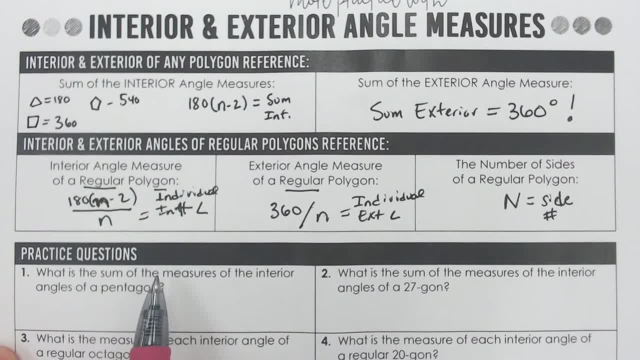 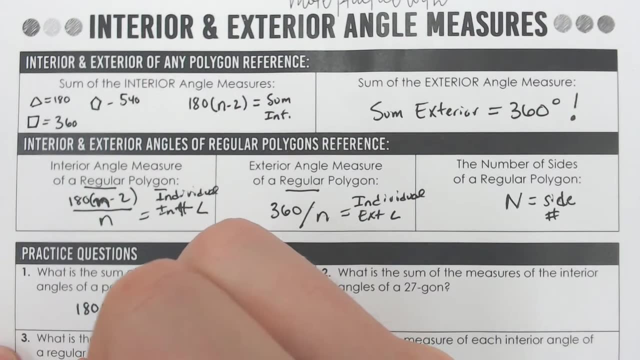 to be able to solve the problems. so what is the sum of the measures of an interior angles of a pentagon? well, a pentagon has five sides, so the sum of the interior angles means my n is going to be 5 and I do 180 times. 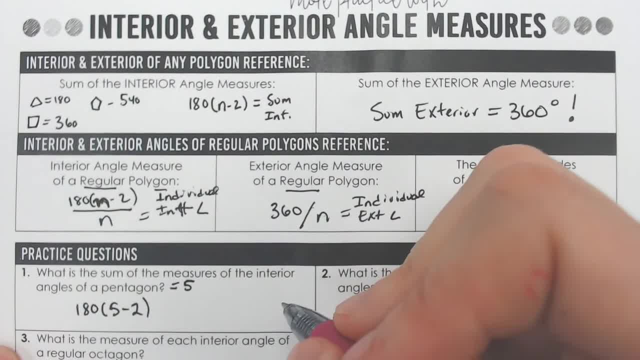 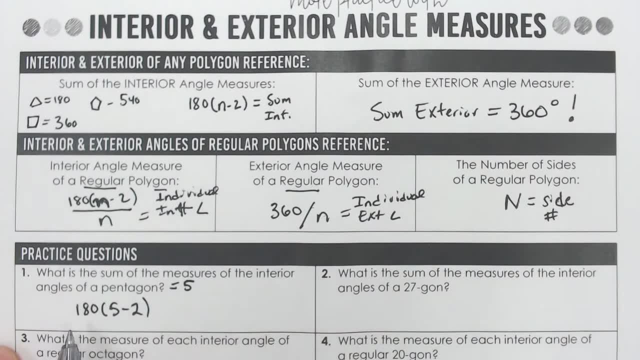 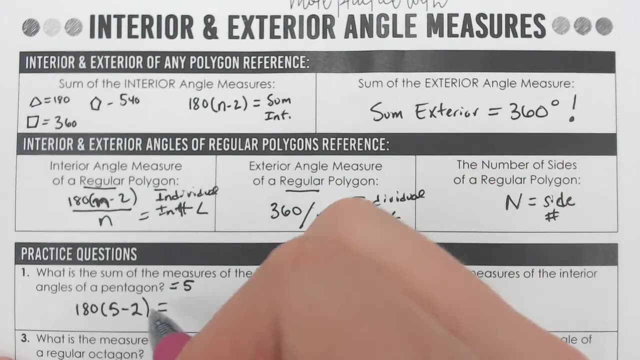 5 minus 2. so I'm going to do 180 times 5 minus 2- sorry for the beeping- and that is going to be what I get. and if I do 180 times 5 minus 2 in my calculator, or 180 times 3, 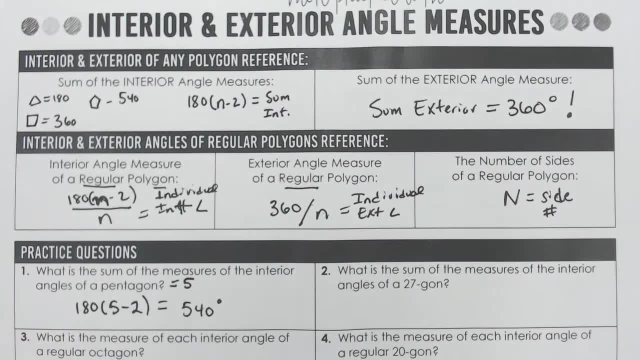 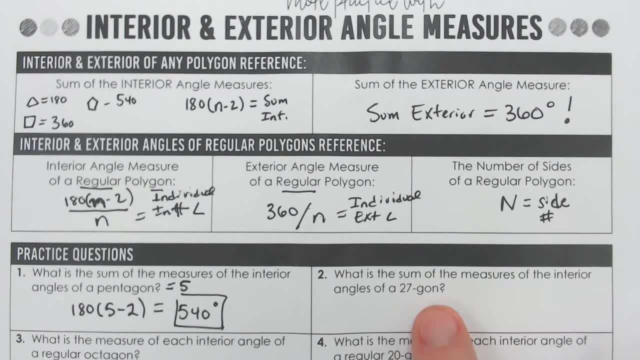 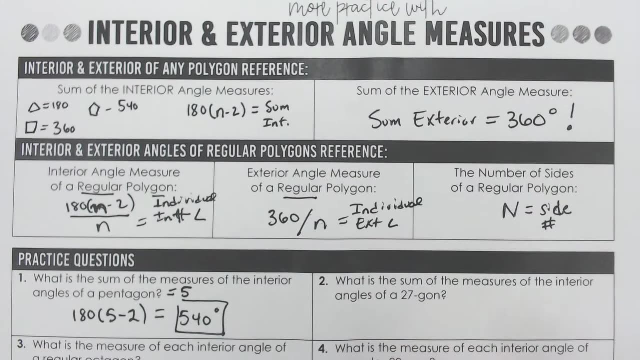 I get 540 degrees and that's it all right now. this next one. this one's going to be a little bit bigger because it's the sum of the measures of the interior angles of a 27 agon. a 27 agon is a lot of sides. that is going to be a very big number, because the more sides you have, the more. 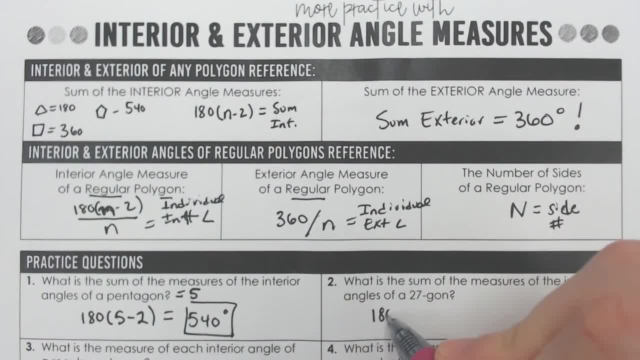 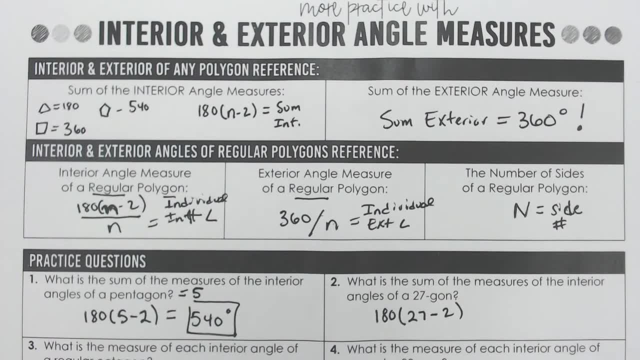 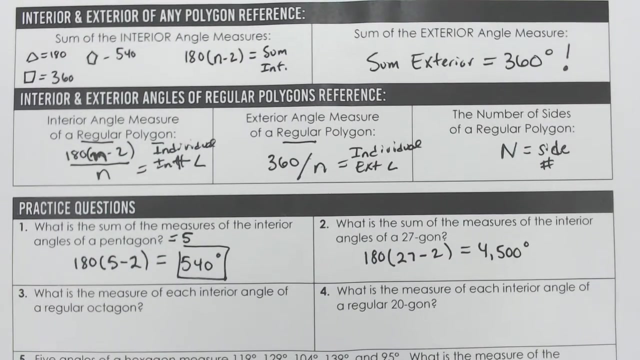 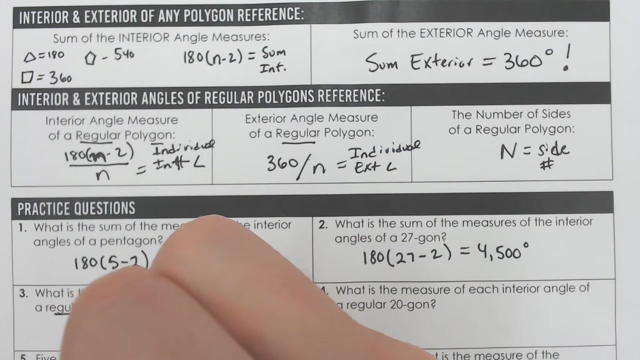 interior angles just keep getting bigger. we have to do 180 times 27 minus 2. I am definitely going to need a calculator for that. 180 times 27 minus 2 or 25 is 4,500 degrees. quite the big number. what is the measure of each interior angle of a regular octagon? well, a regular octagon means that 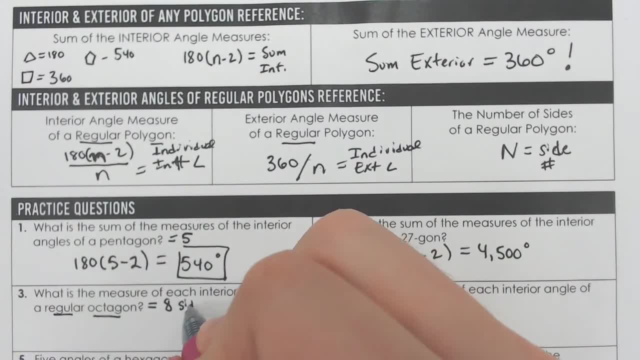 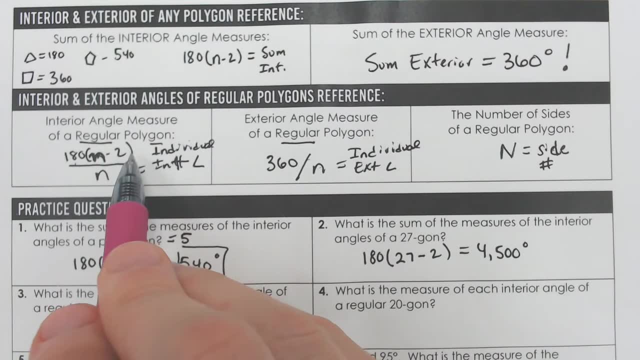 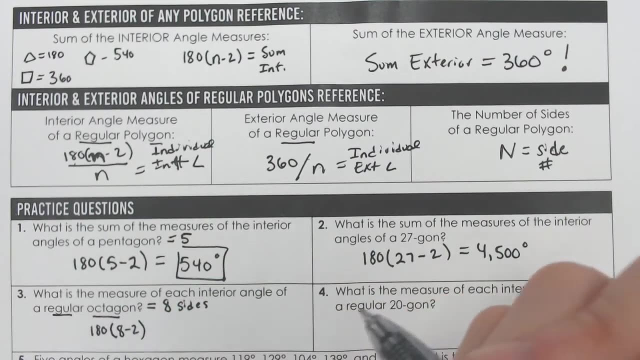 all the sides are equal and an octagon has eight sides to begin with. so what is the measure of each individual angle? So we have to do 180 times 8 minus 2. we're going to get an answer from that and then we're going to. 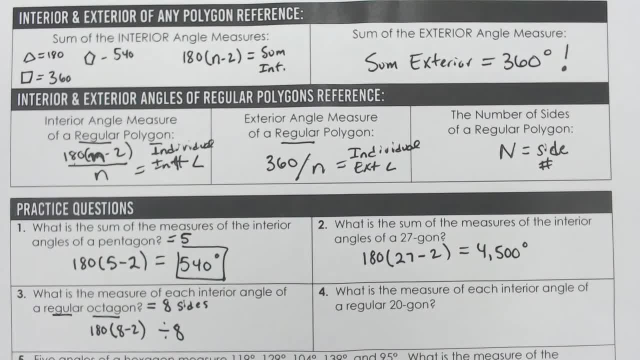 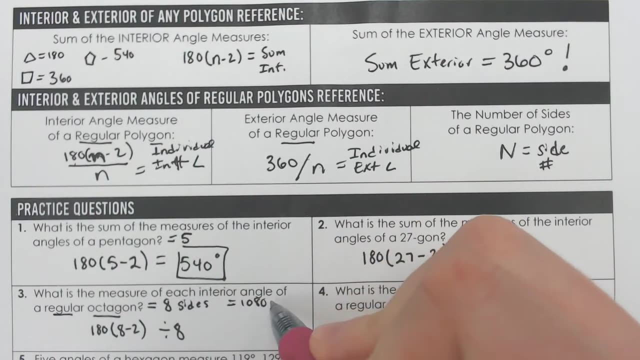 divide that answer by the number of sides, which is 8, so 180 times n minus 2, which is 180 times 8 minus 2, is times 6. you're going to get 1080 from that, which apparently means that the total amount of angles in an octagon is 1080. but we're going to get an answer from that which apparently 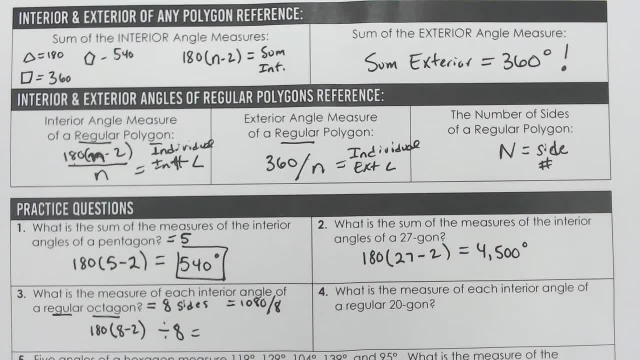 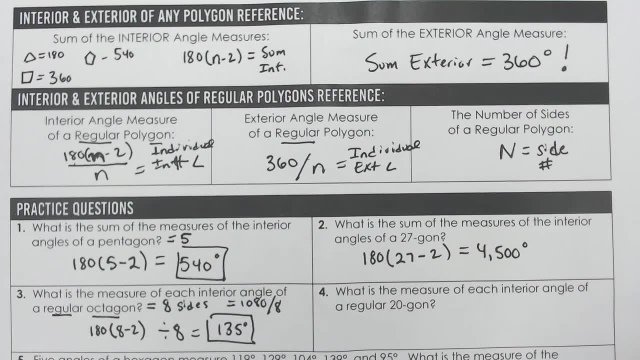 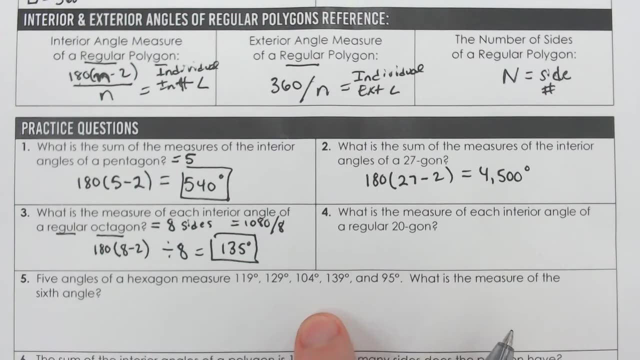 means that the total amount of angles in an octagon is 1080, but you have to divide that evenly by 8 to get the individual, which is 135 degrees. so sometimes they give you some of the angles and you have to find what's missing. what is the angle of the sixth angle? so a hexagon has six sides and 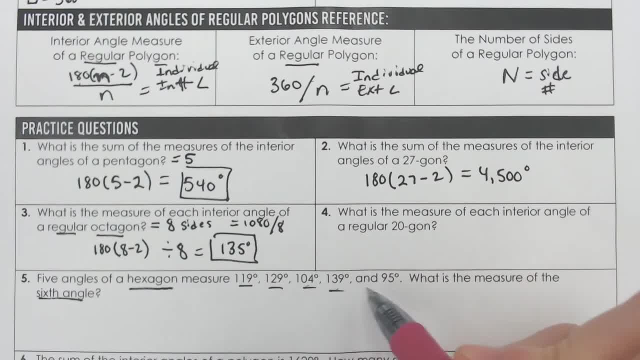 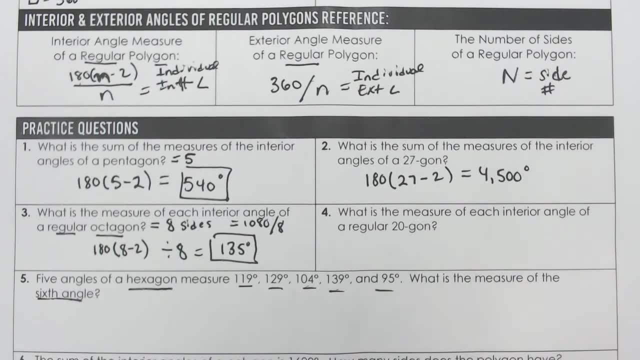 therefore, six angles. we have one, two, three, four, five of them given to us. we're looking for the sixth one. well, in order to do this, I need to know what is the sum of the interior angles of a hexagon. so I'm gonna have to do 180. 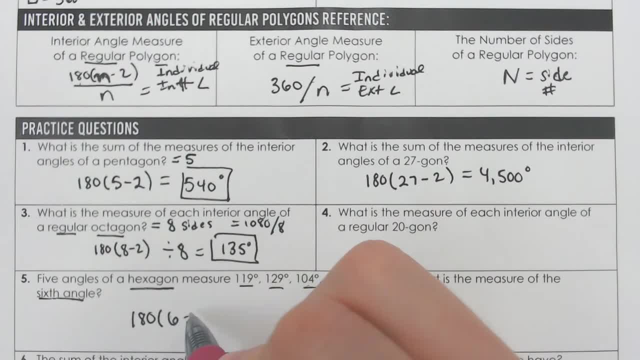 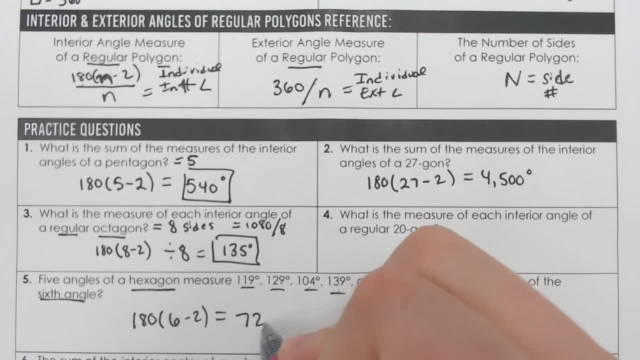 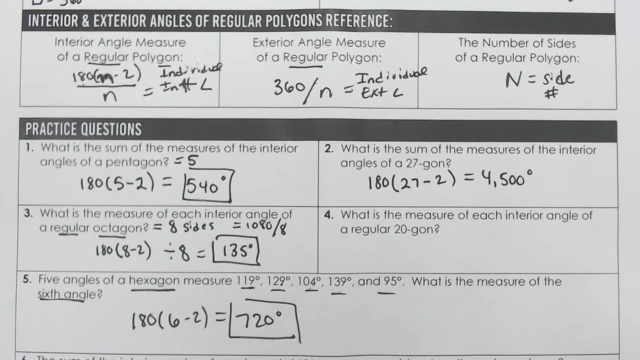 times n minus 2, it's 6 minus 2, and that would be 180 times 4- is equal to 720 degrees. so if all of the angles add to 720- and I already have these- one, two, three, four, five of them- I just have to take these away from 720, so I'm gonna. 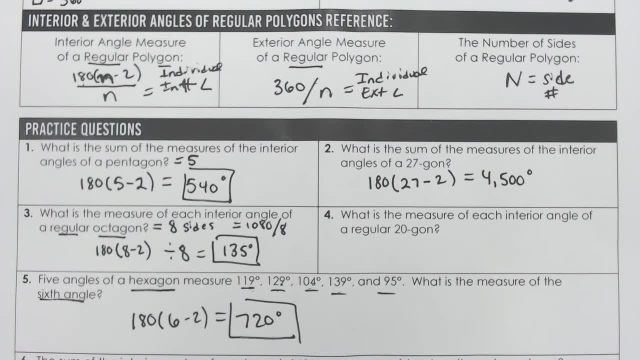 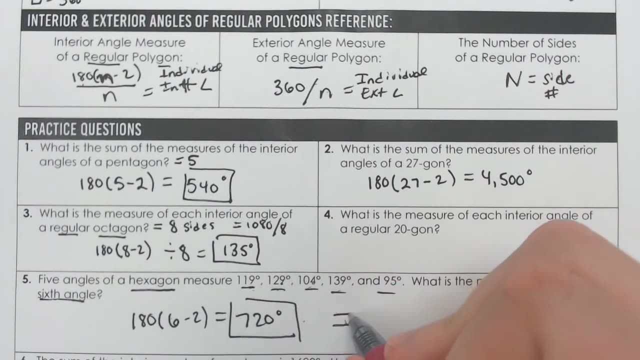 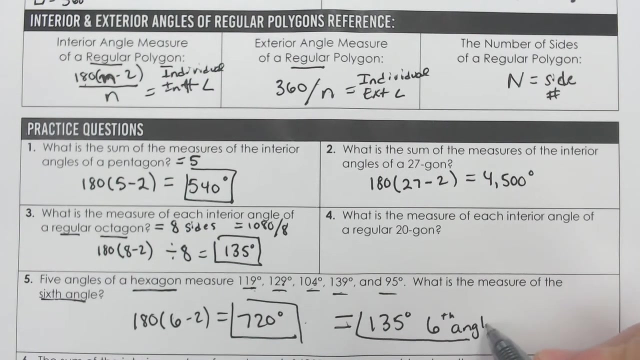 take those away from 720. I'm gonna subtract the 119, I'm gonna subtract the 129, I'm gonna subtract the 104 and the 139 and the 95, all of them away from, so, from 720. if I subtracted all of those, I get 135 degrees left over for that sixth angle, in order for its total. 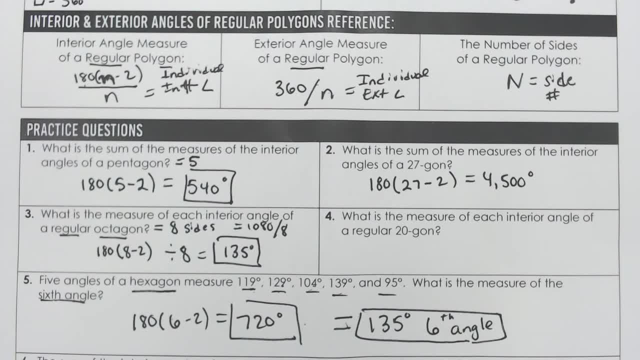 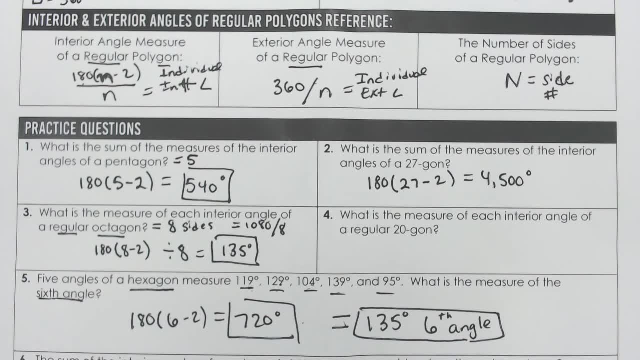 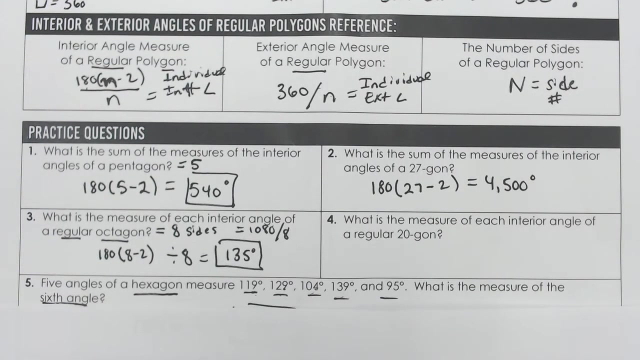 to 720. all right, so that's gonna be how some of the easy problems are. some of the more difficult problems are not any more difficult, but they are on the very high level of annoying factor. okay, so before we do that, I do want to talk about exterior angles a little bit. more. so exterior angles: we haven't talked. about yet other than they have to always add to 360 degrees. so the exterior angle of a regular polygon is 9 degrees. that means that each and every exterior angle is 9 degrees. how many sides does it have? Well, always, the exterior angles always add to. 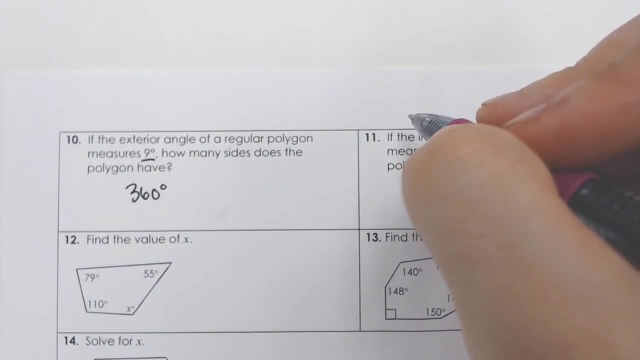 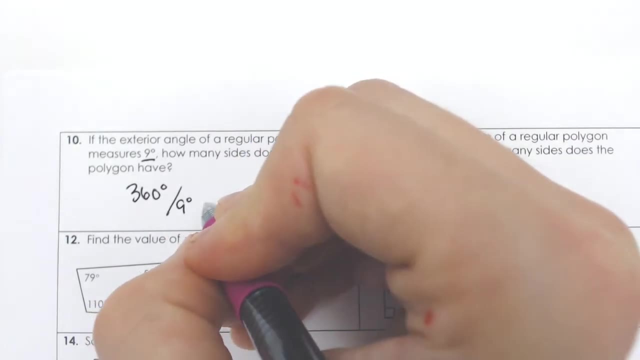 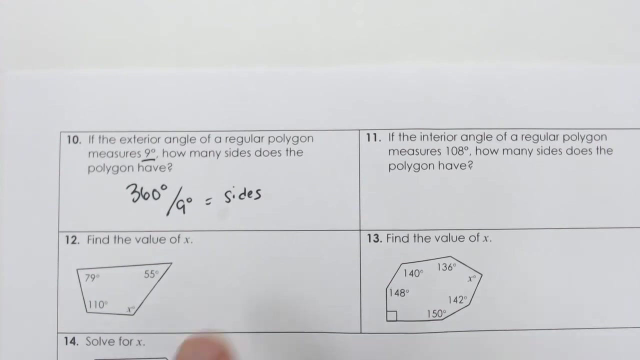 360.. Okay, so if all of the exterior angles on this regular polygon add to 360, I can just divide that by 9 and I'll get the number of sides. You can always divide 360 by the number of sides or the angle of each one to get the sides. It doesn't matter, it's. 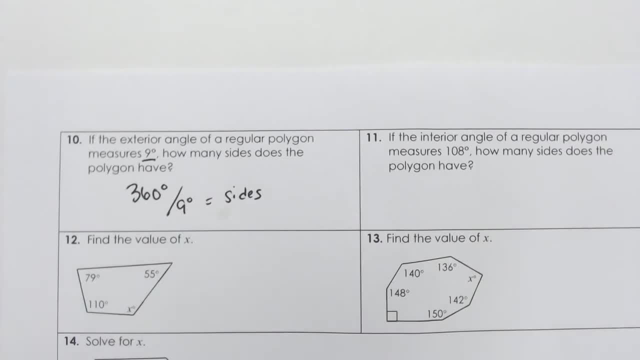 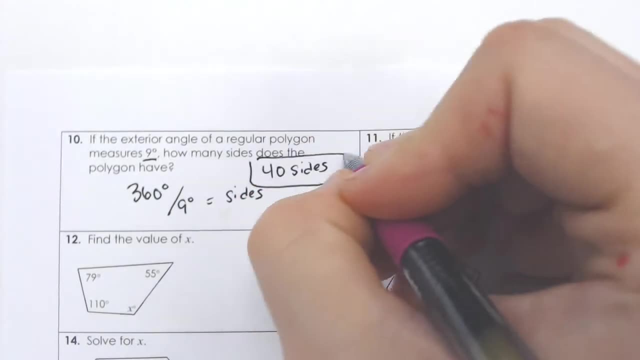 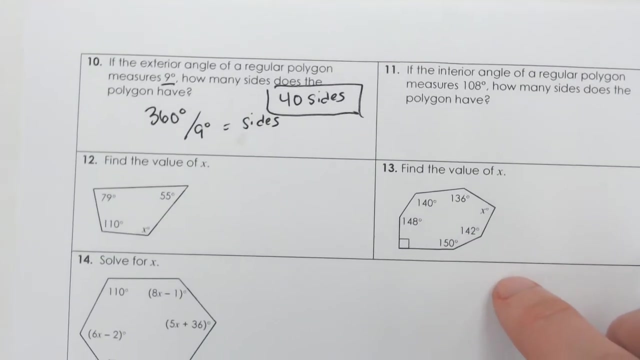 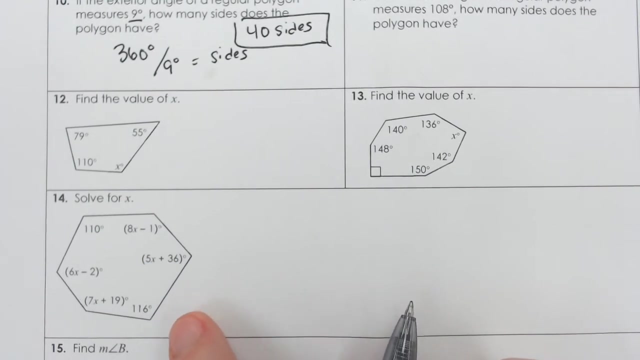 just 360 divided every time. So 360 divided by 9 is 40 sides. Good grief, that's a lot of sides. Alright, and now, without further ado, we get the problems that nobody likes to do, and that's these. They're not any harder, but apparently this is too easy of a concept. 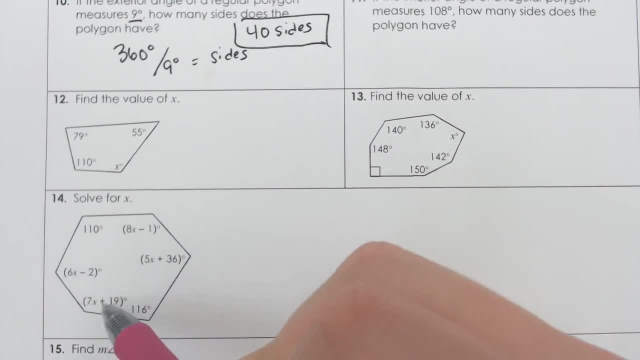 so occasionally, some teachers, including myself, like to make an equation that is, without a better word, very long and hard to do. potentially Either way, we have to figure out how many sides we have here. We have 1,, 2,, 3,, 4,, 5,. 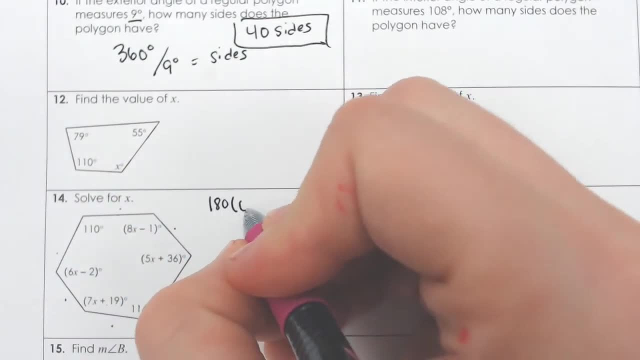 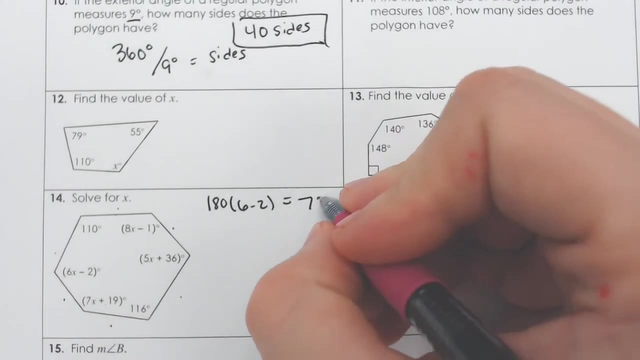 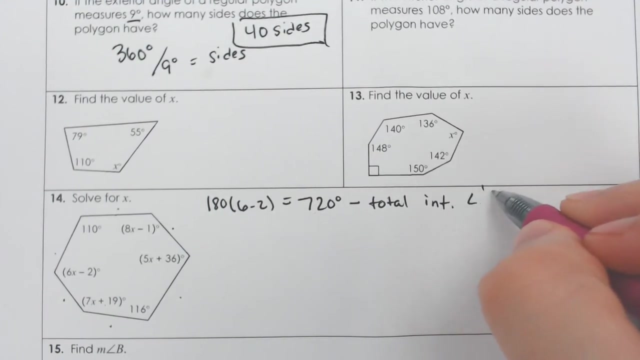 6 sides. so we have to do 180 times 6 minus 2 to get the total interior angles, And in this case it's 720 degrees. That is the total interior angles. So that means if I were to add up all these angles it equals 720.. So we've done these. 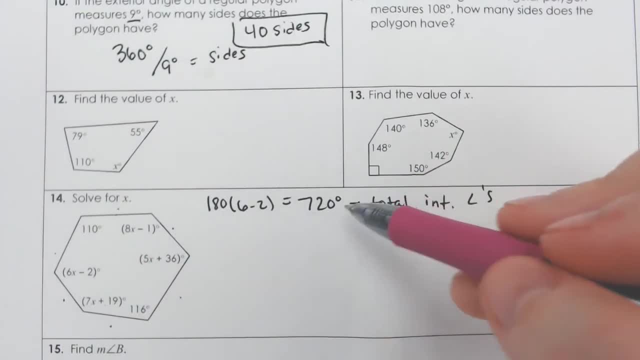 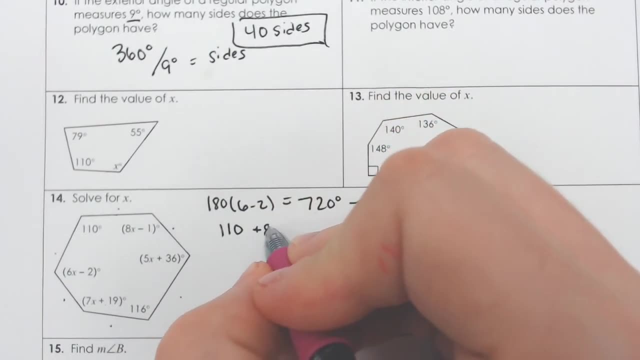 with triangles, where you have to add up all the angles to equal 180, now it's just not equal to 180,, it equals 720. And you have a lot to add. We have to do 110, and 8x minus.